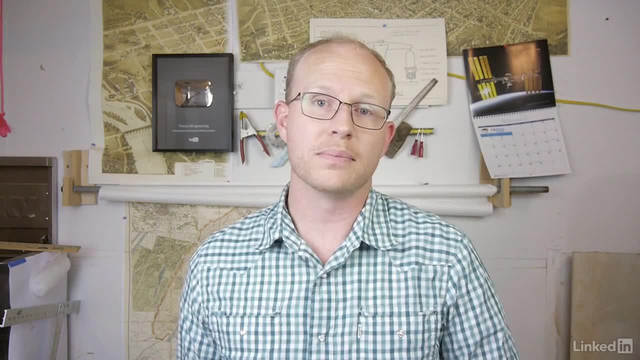 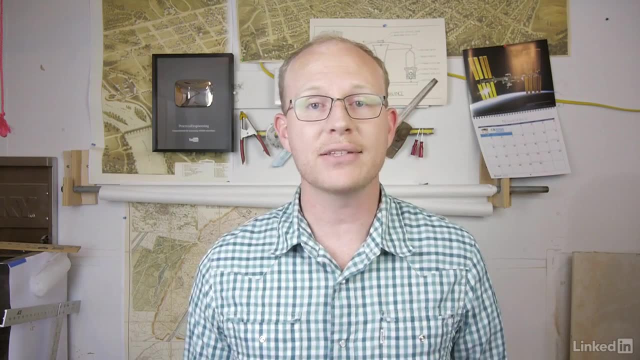 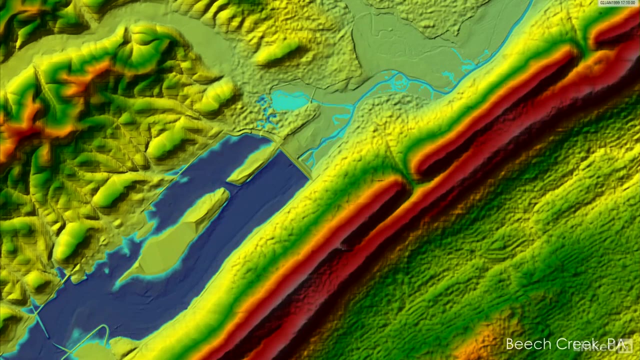 website and download RAS for yourself. but why would you No, seriously? why do we care about river hydraulics and what are the questions that engineers try to answer with a model of a river system? Let's use RAS to find out. And, by the way, most of the demonstrations in this video are: 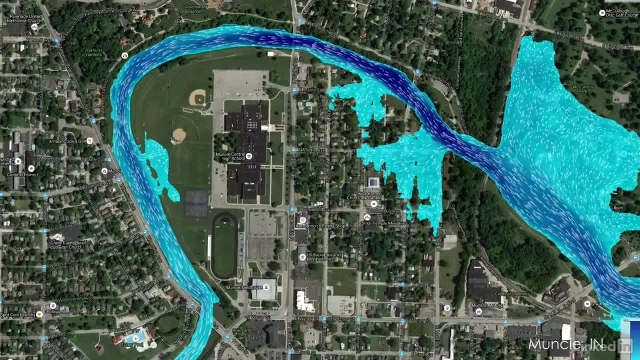 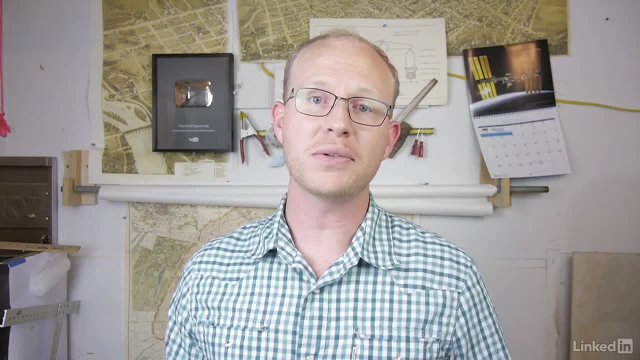 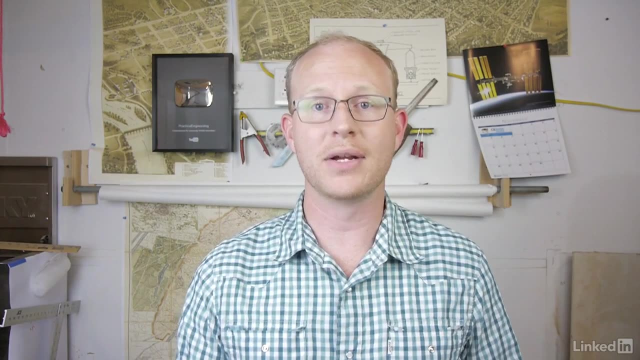 from example data that ships with the software. The places are real, but the situations are not. My apologies in advance if you live in Muncie. The number one use of hydraulic river models is to estimate flooding. For riverine flooding engineers can follow a drop of water from inside a storm cloud. 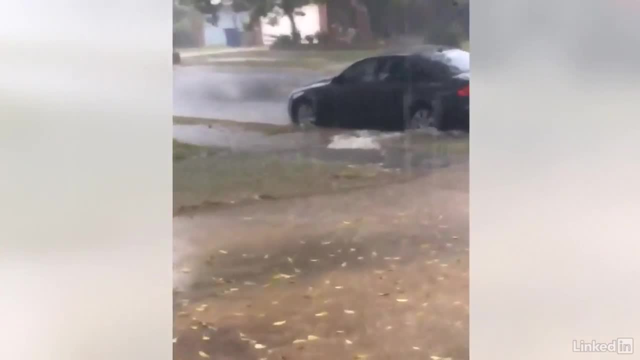 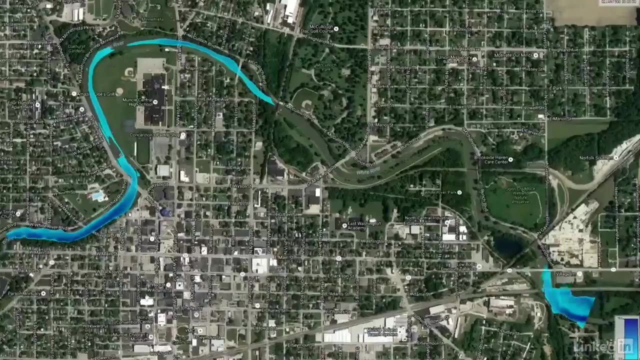 to inside someone's house. First you have to know how much rain falls and how much of that rain makes its way into the creeks and rivers. That's hydrologic analysis. Once you know how much water enters a river, you need a hydraulic model to find out how much. 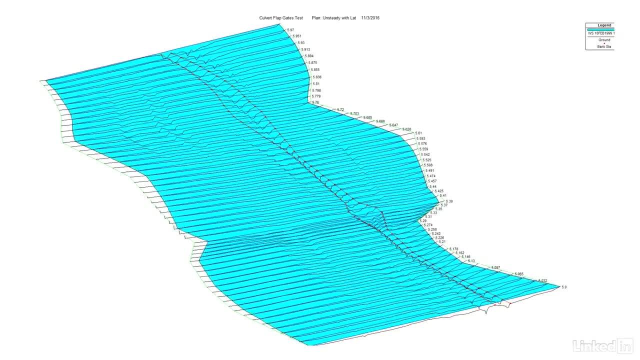 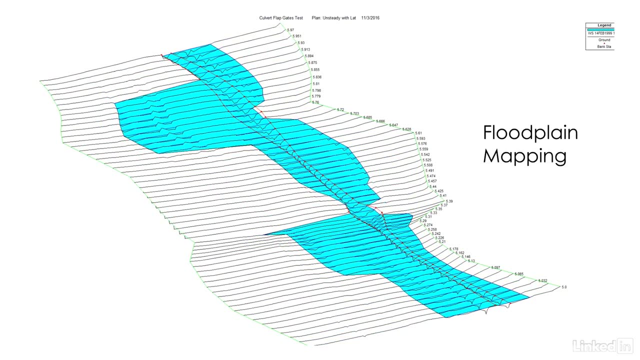 the river rises as a result. This process is called floodplain mapping, and it helps us characterize which areas are at the highest risk of flooding, so that we can be prepared when and if it happens. Another way we can use models is to evaluate projects. 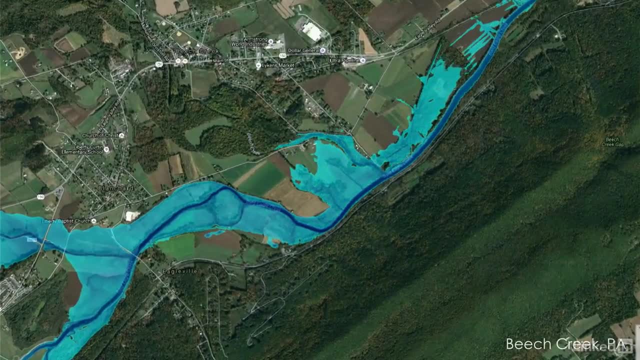 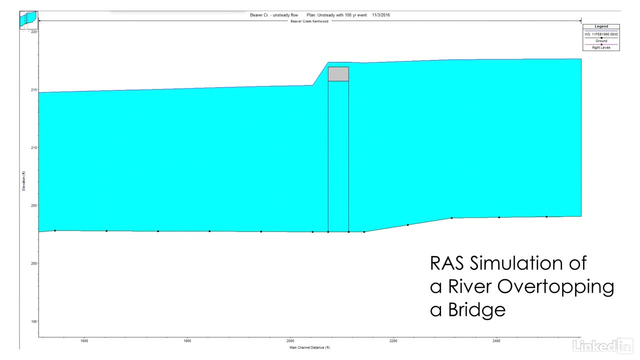 Putting a levee on a river may help flooding in one location, but make it worse. downstream Models help to represent a real world situation without the cost and complexity of actually performing a test at full scale. Obviously, we can't create a flood just to see what happens. so models allow us to test. 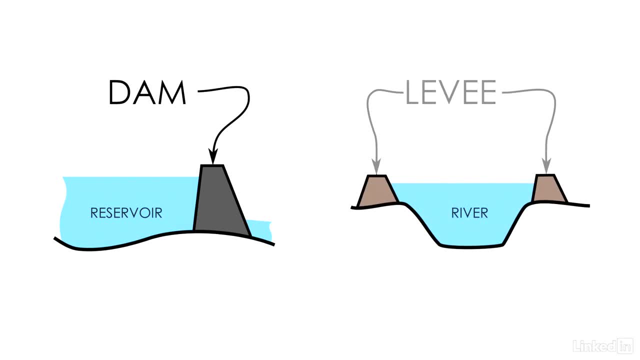 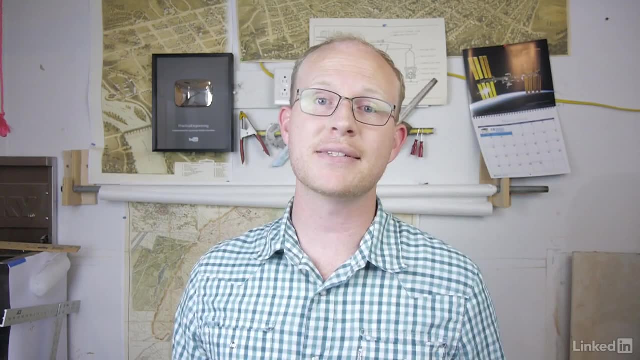 out hydraulic structures like dams and levees, to make sure they work as anticipated, before spending millions of dollars on construction. Another use of hydraulic models is simulating systems of reservoirs, When you have a number of dams along a river, all with different operating guidelines and 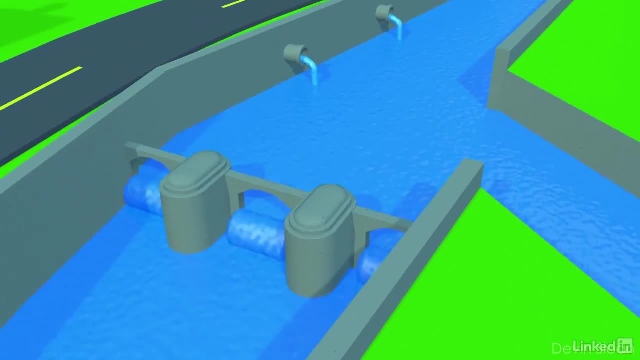 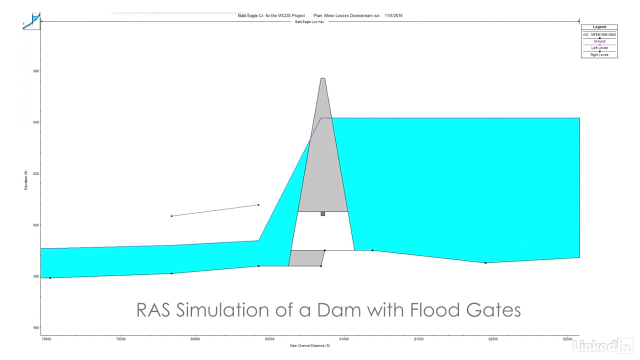 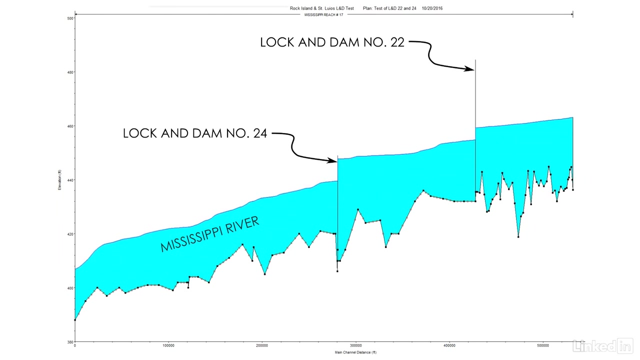 all trying to accomplish different objectives, like water supply, navigation and flood control. things get complicated in a hurry. A hydraulic river model can perform simulations of these complex scenarios to help with planning and optimization of operations. For example, this model shows how two 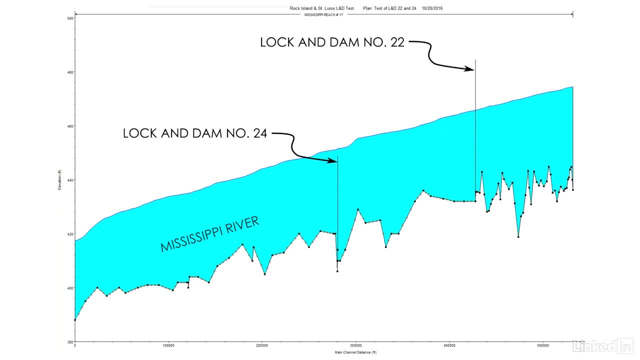 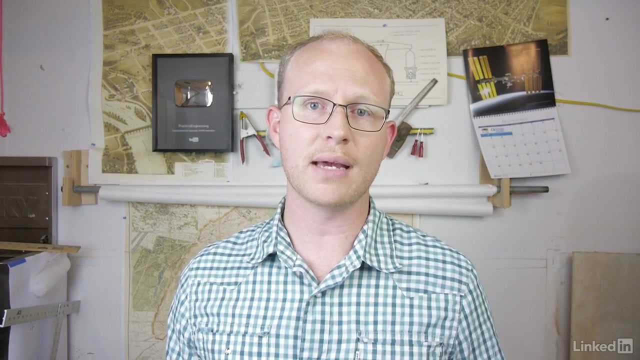 now, navigation dams on the Mississippi River manage the locks and gates during a flood situation. A model can also be predictive, helping operators anticipate conditions before they even happen. Finally, we use hydraulic models to perform breach analyses for dams. If a dam fails, it can release a tremendous amount of water in a short period of time. 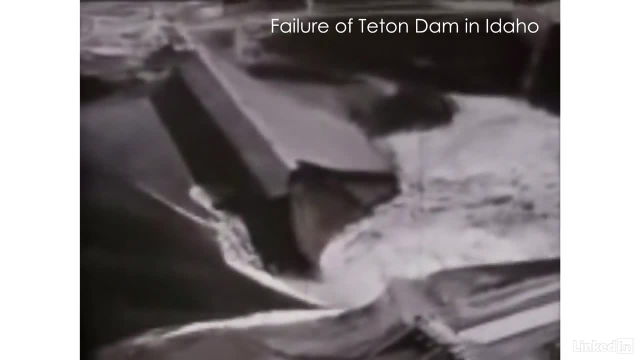 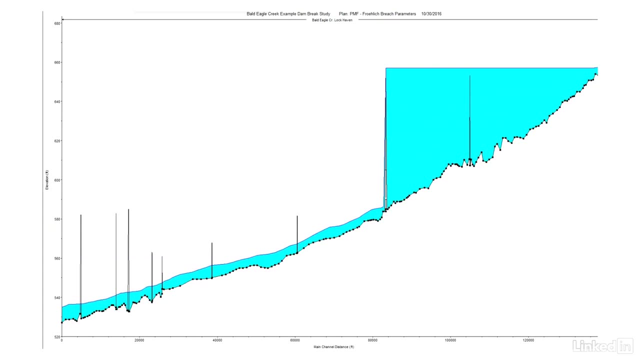 In fact, some of the worst engineering disasters in history have been dam failures. In situations like this, emergency managers don't have much time to react, so many dams are required to have emergency action plans. Part of these plans is mapping out the areas that might be affected in the event of a breach. 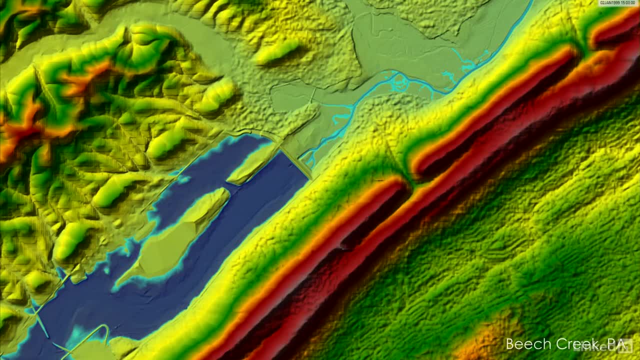 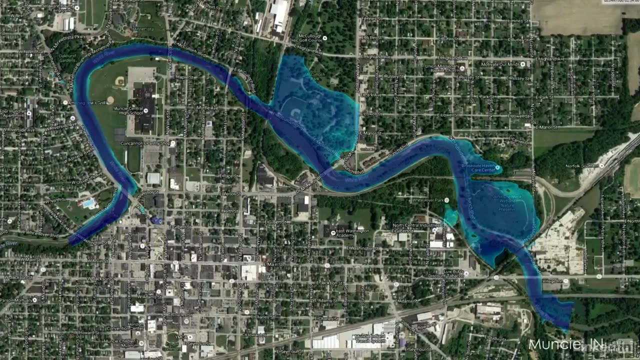 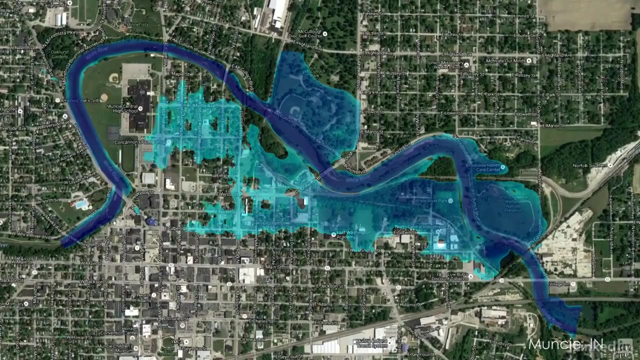 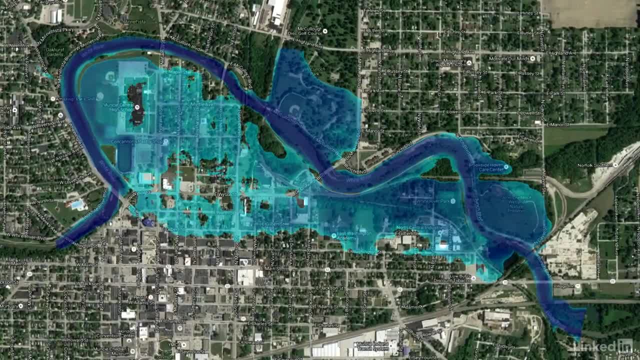 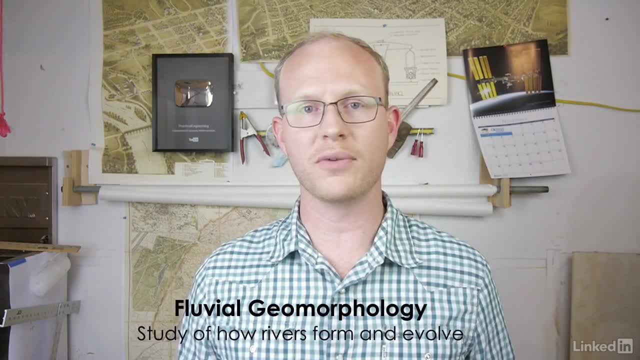 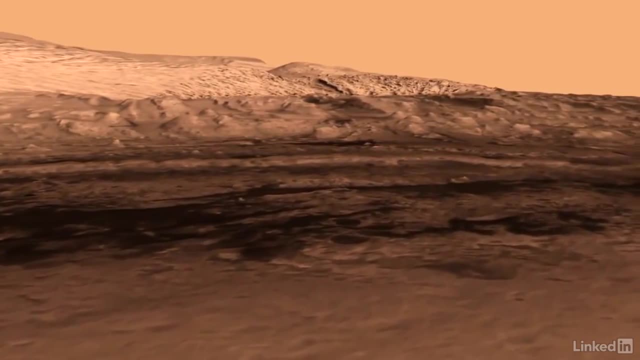 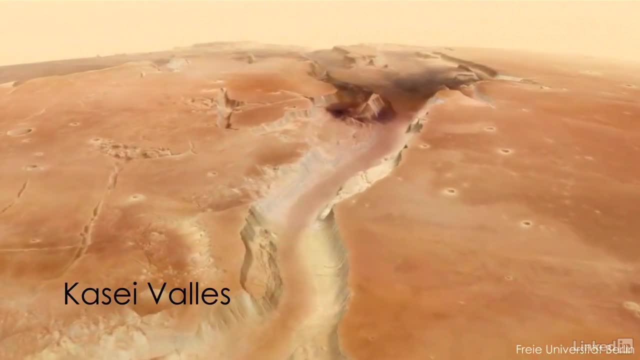 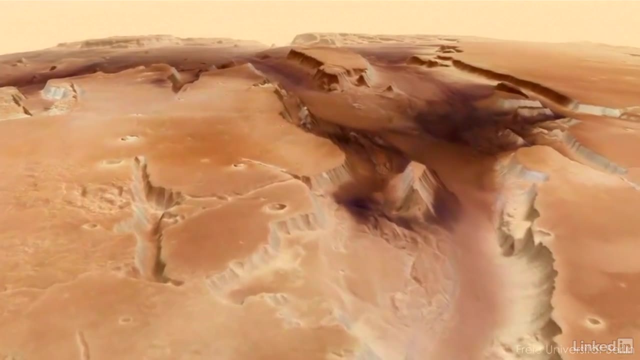 red neighbor Mars. The Casei Vallis is one of the largest outflow channel systems on Mars-almost twenty times the width of the Grand Canyon and several kilometers deep �를. Scientists believe that billions of years ago, liquid water may have flowed on the surface. 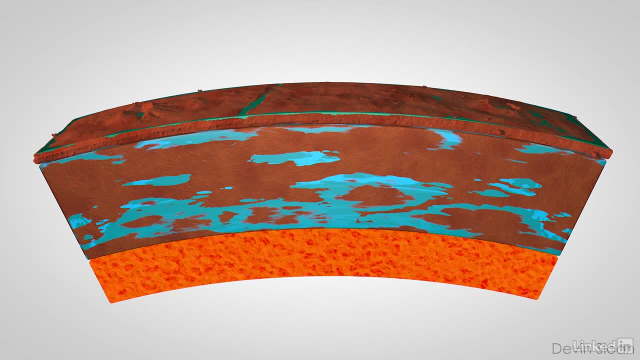 and in underground aquifers on Mars. As the planet cooled, the water on the surface froze, creating an impermeable cap to a deep layer of pressurized liquid groundwater, just like the top to a bottle of soda. Scientists think that tectonic movement or volcanic activity 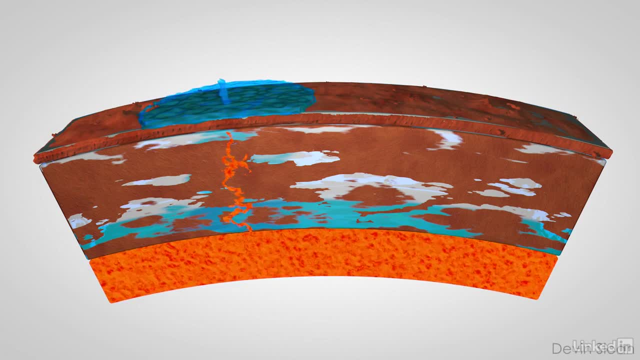 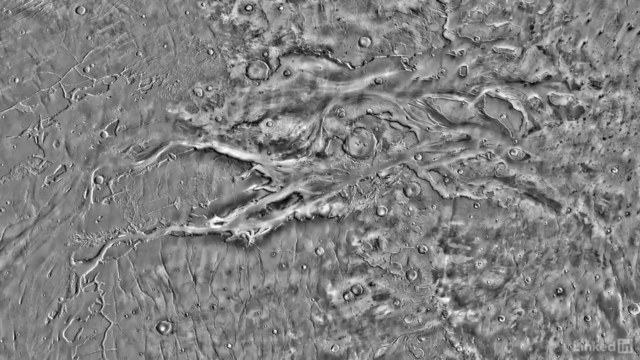 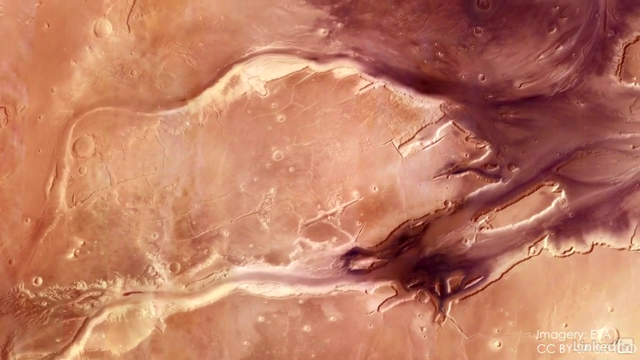 may have melted the subsurface ice, popping the top on the cryosphere and releasing a massive flood wave of pressurized groundwater. These massive floods are what likely created many of Mars' outflow channels like the Kisei Valles. But what's an Earth-bound geomorphologist to do?